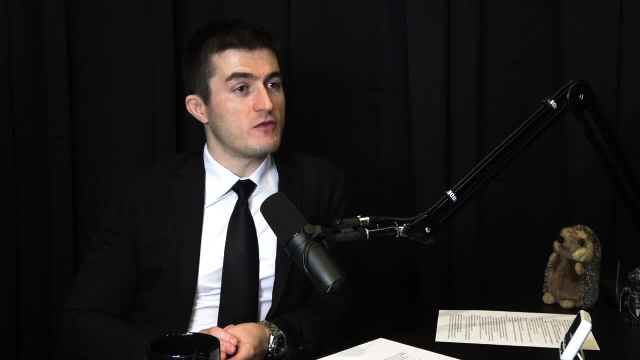 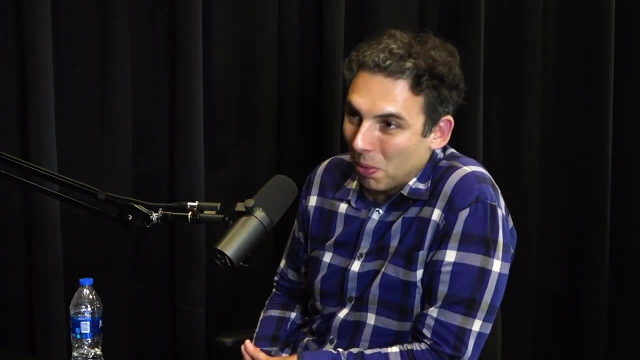 about doing work in artificial intelligence and robotics and are thinking about whether to get a PhD. I was at CMU for undergrad as well and didn't know anything about robotics, coming in and was doing electrical computer engineering, computer science, and really got more and more. 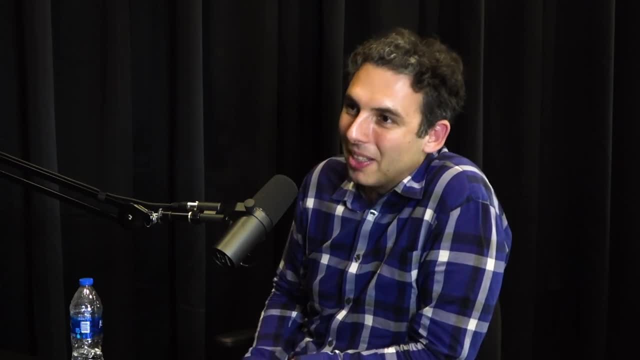 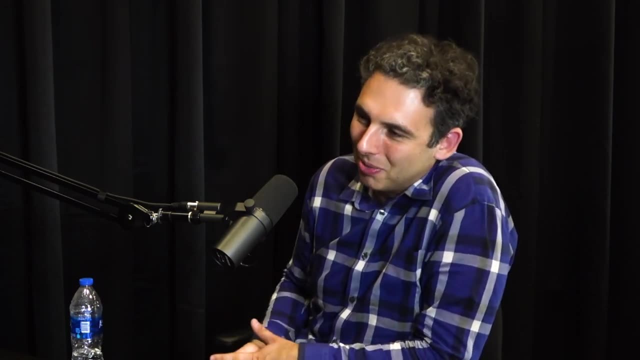 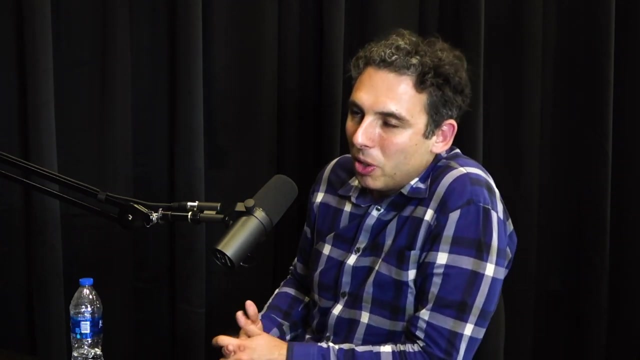 into AI and then fell in love with autonomous driving, And at that point, that was just by a big margin, such an incredible central spot of investment in that area, And so what I would say is that robotics- for all the progress that's happened- is still a really young field. There's a huge amount of 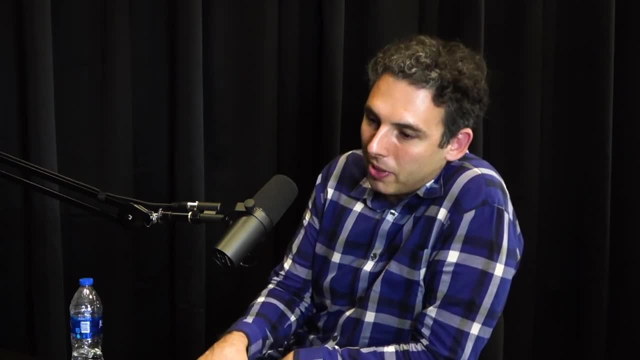 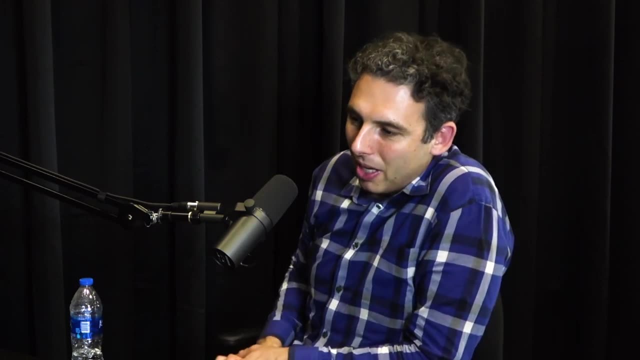 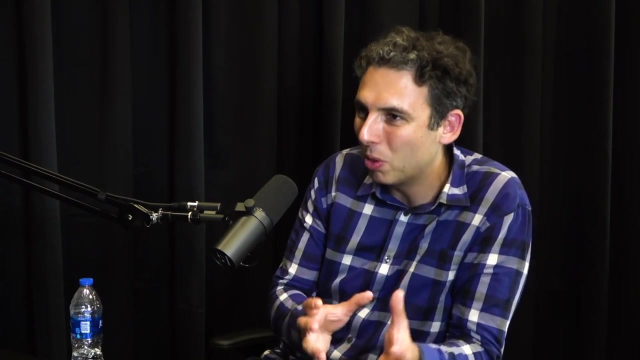 opportunity. Now that opportunity shifted where something like autonomous driving has moved from being very research and academics driven to being commercial driven, where you see the investments happening in commercial. Now there's other areas that are much younger and you see grasping at an impelation, making the same sort of journey that autonomy made. and there's other areas as 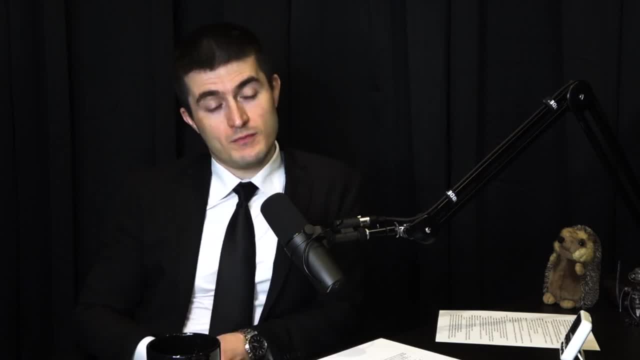 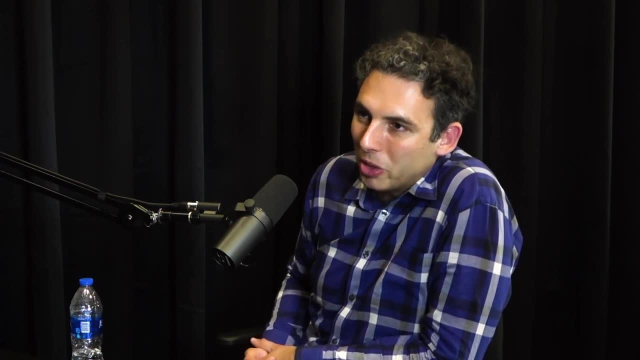 well, What I would say is: the space moves very quickly. Anything you do a PhD in, like it is in most areas, will evolve and change as technology changes and constraints change and hardware changes and the world changes, And so the beautiful thing about robotics is it's super. 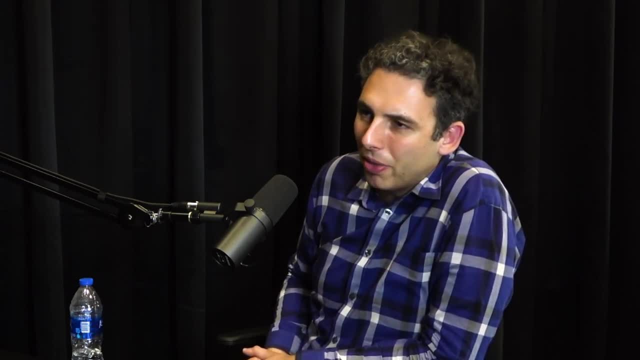 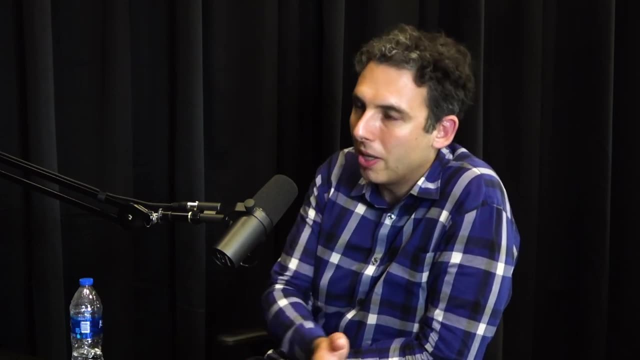 broad. It's not a narrow space at all and it can be a million different things in a million different industries, And so it's a great opportunity to come in and get a broad foundation on AI, machine learning, computer vision systems, hardware sensors- all these separate things. 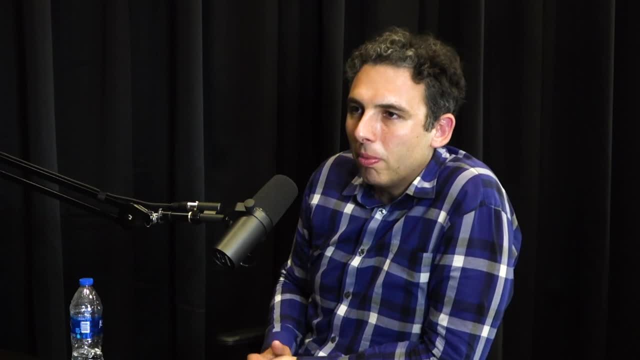 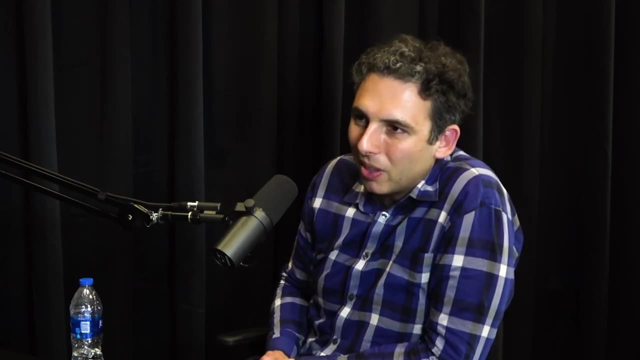 You do need to go deep and find something that you're like really, really passionate about. Obviously, just like any PhD, this is like a five, six year kind of endeavor And you have to love it enough to go super deep to learn all the things. 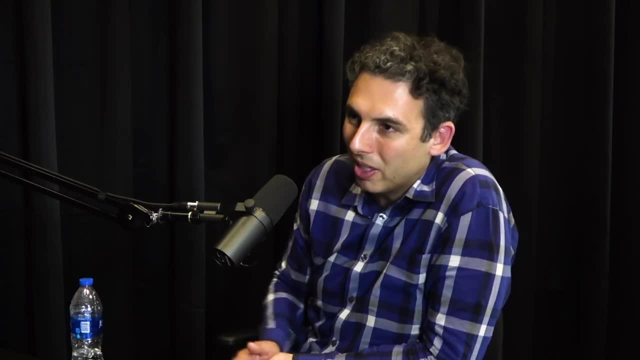 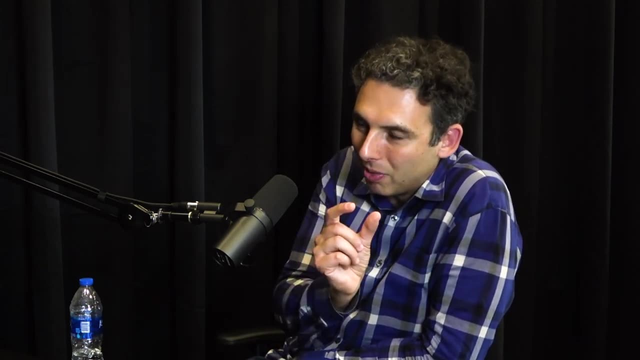 necessary to be super deeply functioning in that area and then contribute to it in a way that hasn't been done before. And in robotics that probably means more breadth, because robotics is rarely kind of like one particular kind of narrow technology, And it means being able to collaborate. 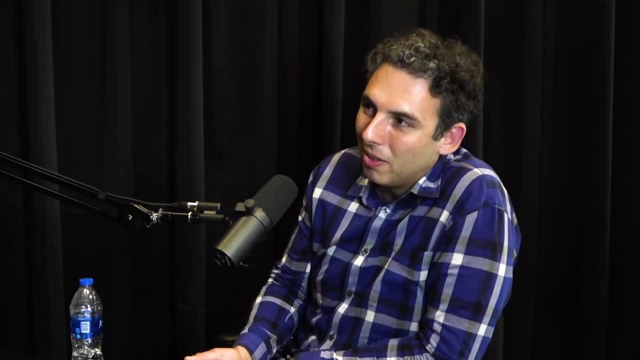 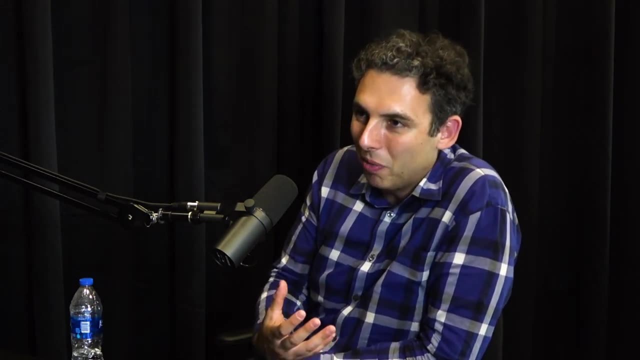 with teams where, like you know, you can do a lot of things, And I think that's a really like. one of the coolest aspects of like the experience that I like kind of cherish in our PhD is that we actually had a pretty large AV project that for that time was like a pretty 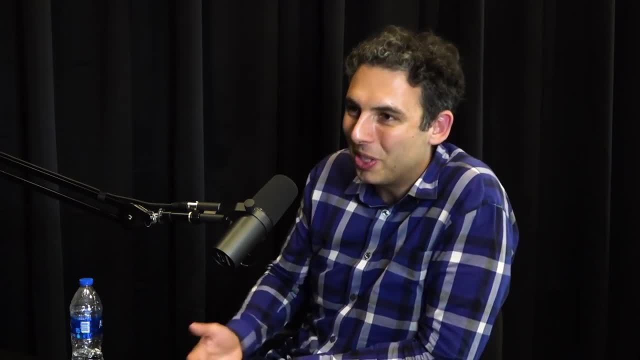 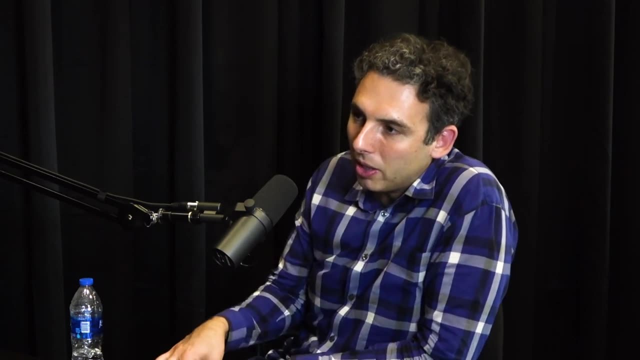 serious initiative where you got to like partner with a larger team and you had the experts in perception and the experts in planning and the staff and the mechanical engineers. It was a DARPA challenge. So I was working on a project called UPI back then, which was basically the off-road version. 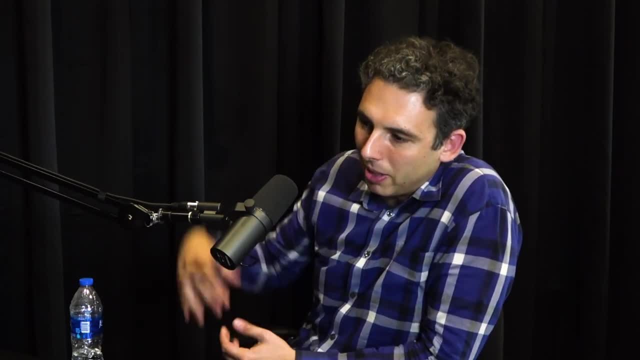 of the DARPA challenge. It was a DARPA funded project- for basically, like a large off-road vehicle that you would like drop and then give it a waypoint 10 kilometers away and it would have to navigate a completely unstructured environment. 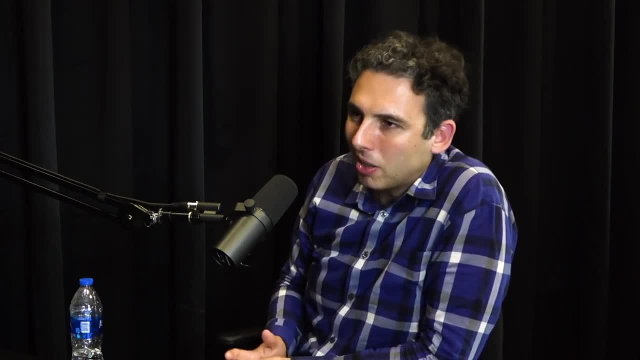 In an off-road environment, Yeah, So like forests, ditches, rocks, vegetation, And so it was like a really really interesting kind of a hard problem where, like wheels, would be up to my shoulders It's. 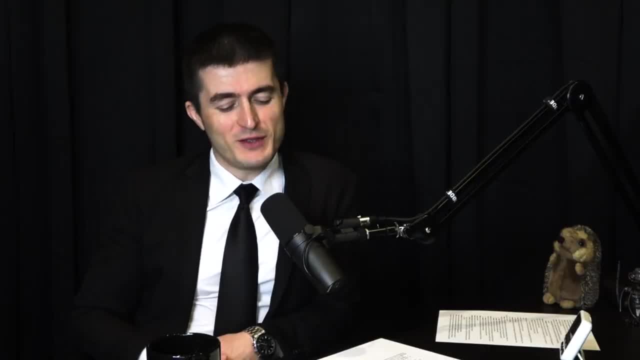 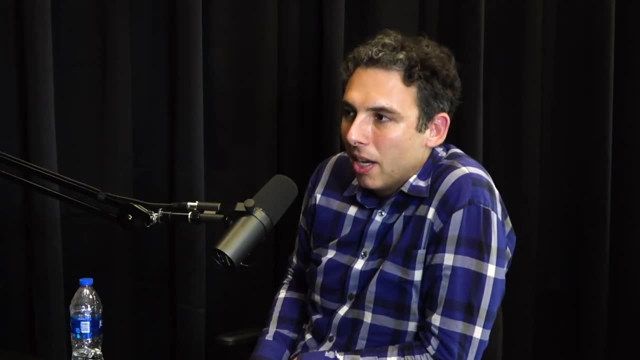 like gigantic right. Yeah, By the way, AV for people stands for autonomous vehicles. Autonomous vehicles, yeah, Sorry. And so what I think is like the beauty of robotics, but also kind of like the expectation, is that there's spaces in computer science where you can. 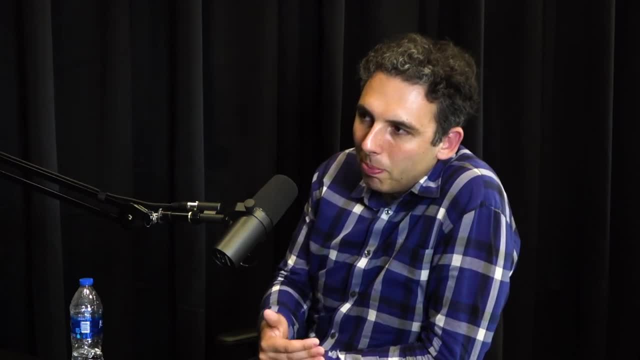 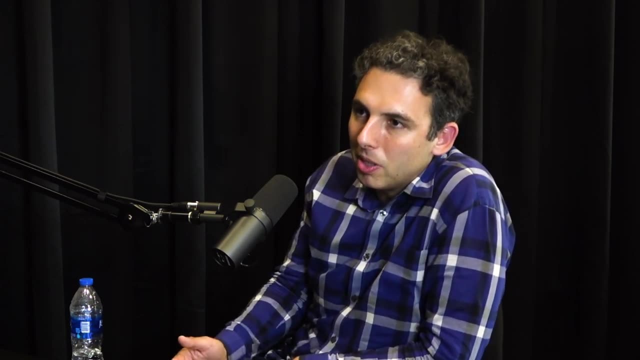 be very, very narrow and deep Robotics. one of the necessity, but also the beauty of it, is that it forces you to be excited about that breadth and that partnership across different disciplines that enable it. But that also opens up so many more doors where you can go and you can do robotics in almost any category. 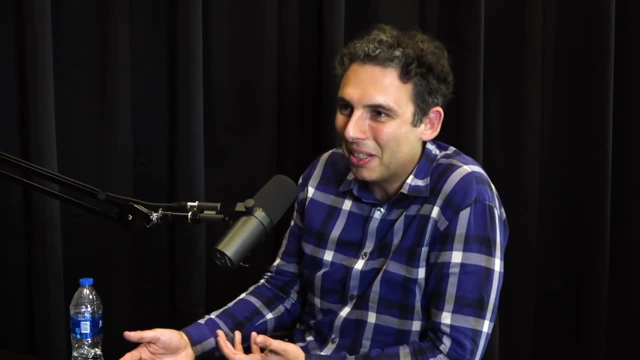 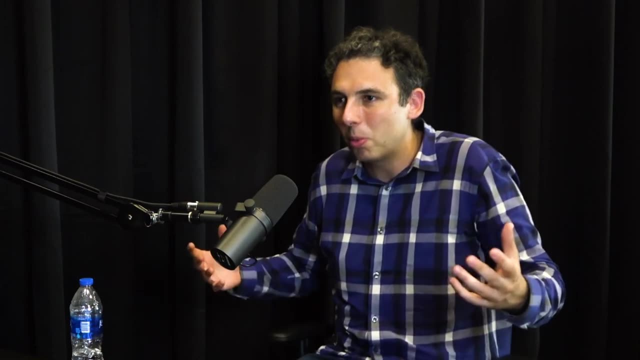 where robotics isn't really an industry. It's like AI, right? It's like the application of physical automation to, you know, to all these other worlds, And so you can do robotic surgery, you can do vehicles, you can do factory automation. 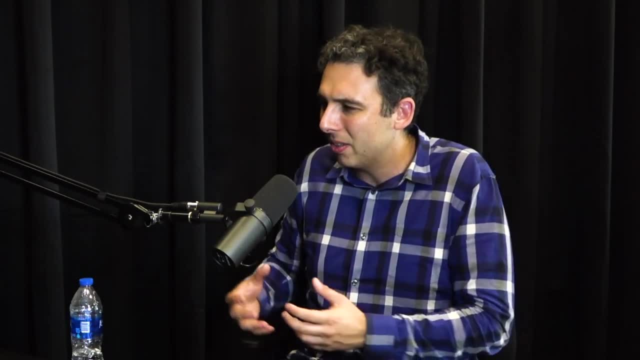 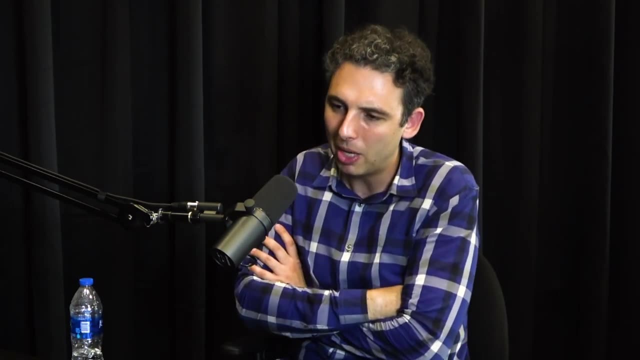 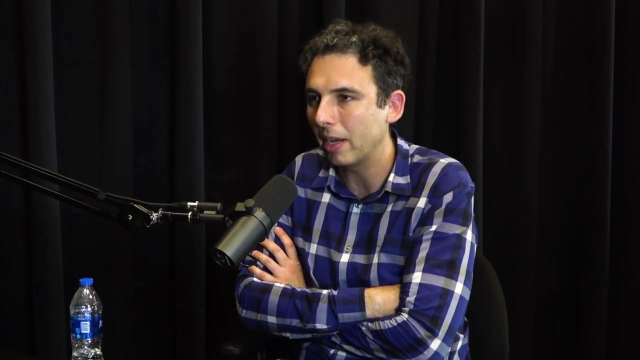 You can do healthcare, you can do like, leverage the AI around the sensing to think about static sensors and scene understanding. So I think that's got to be the expectation and the excitement And it breeds people that are probably a little bit more collaborative and more excited about. 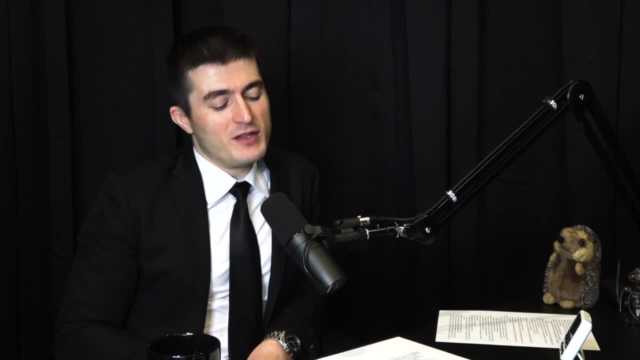 working in teams. If I could briefly comment on the fact that the robotics people I've met in my life, from CMU and MIT- they're- They're really happy people because I think it's the collaborative thing I think you don't. 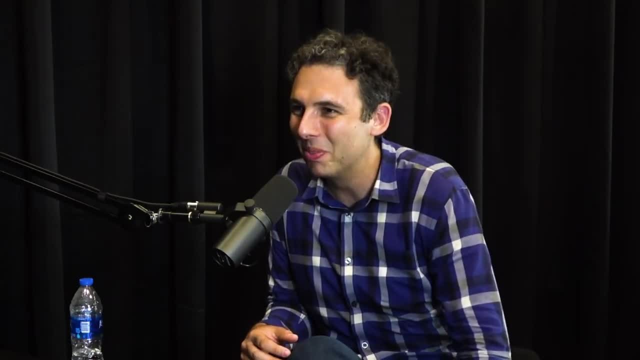 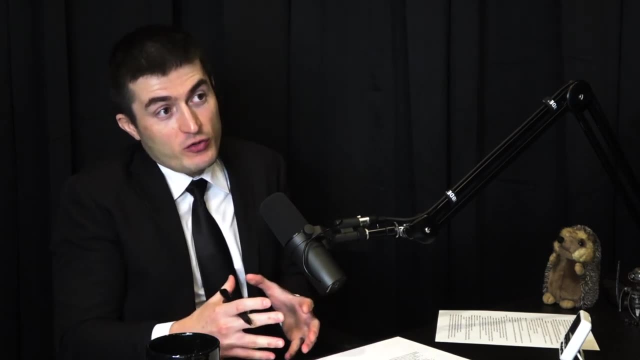 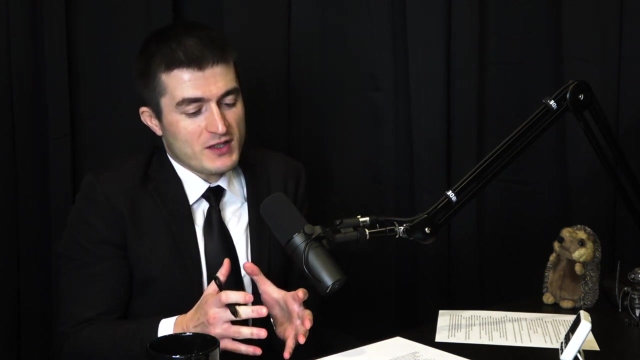 You're not like sitting in like the fourth basement. Yes, exactly When you're doing machine learning, purely software, it's very tempting to just disappear into your own hole and never collaborate And that breeds a little bit more of the silo mentality of like I have a problem. It's almost like negative to. 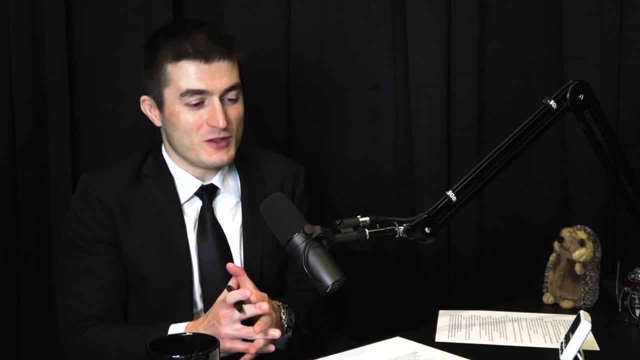 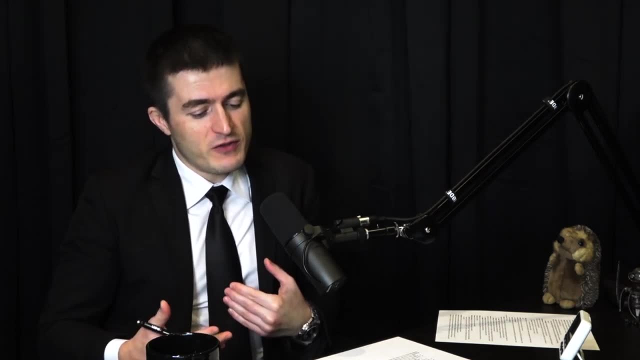 talk to somebody else, Yeah, Or something like that. But robotics- folks- are just very collaborative, very friendly and just, And there's also an energy of like you get to confront the physics of reality often, which is humbling and also exciting. So it's humbling when it fails and exciting when 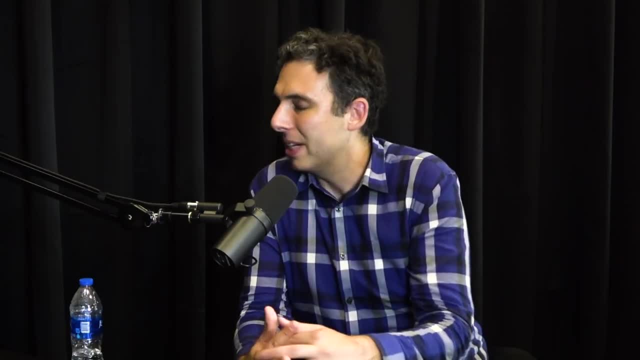 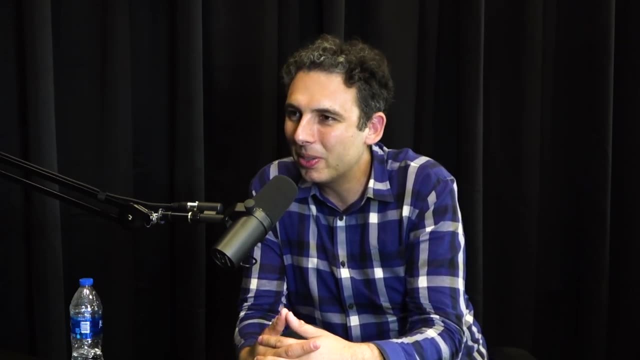 it finally works. It's like a purity of the passion. You've got to remember that, like right now, like robotics and AI is like just all the rage and autonomous vehicles and all this Like 15 years ago and 20 years ago. 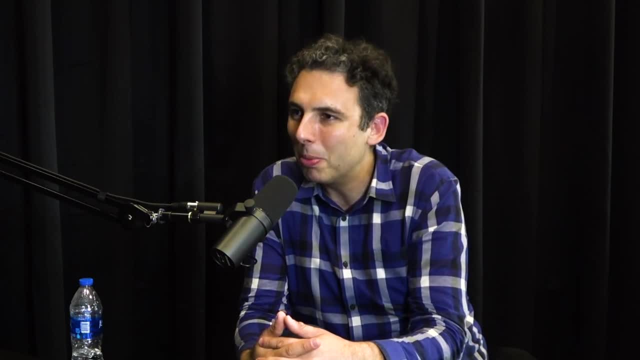 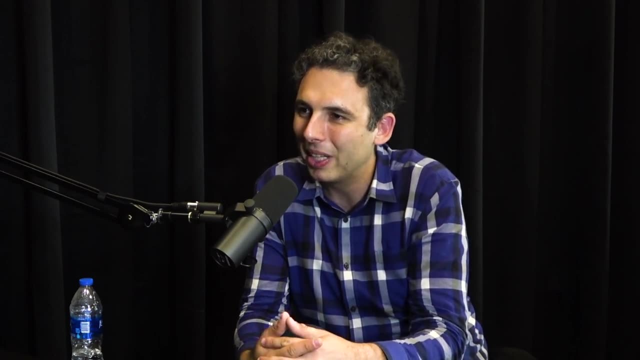 Yeah, it wasn't that deeply lucrative People that went into robotics. they did it because they thought it was just the coolest thing in the world to make physical things intelligent in the real world, And so there's a raw passion where they went into it for the right reasons. 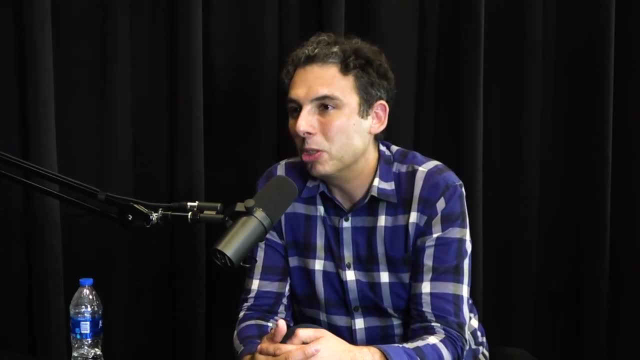 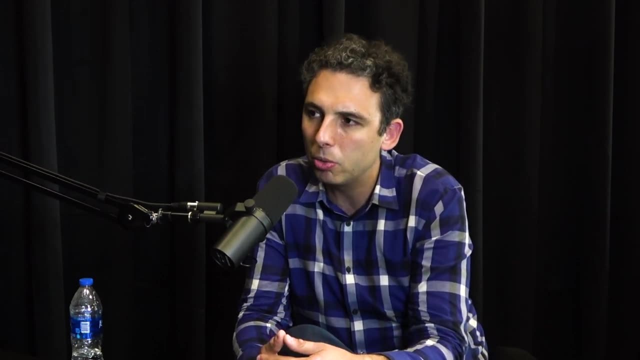 and so forth, And so it's a really great space. And that organizational challenge. by the way, when you think about the challenges in AV, we talk a lot about the technical challenges. The organizational challenge is through the roof where you think about what it takes to build an. 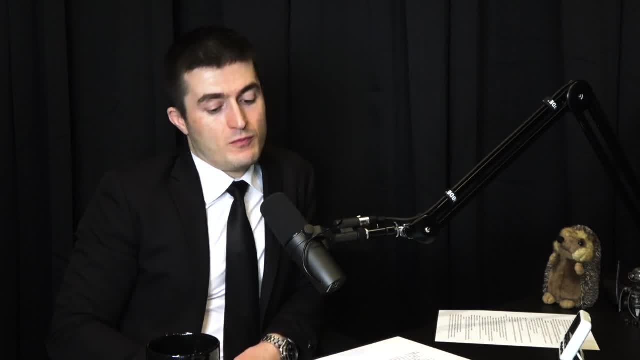 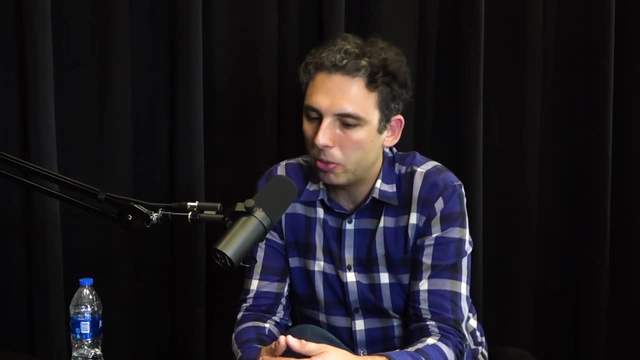 AV system And you have companies that are now thousands of people And you know you look at other really hard technical problems like an operating system. it's pretty well established, Like you kind of know, that there's a file system, there's virtual memory, there's this. 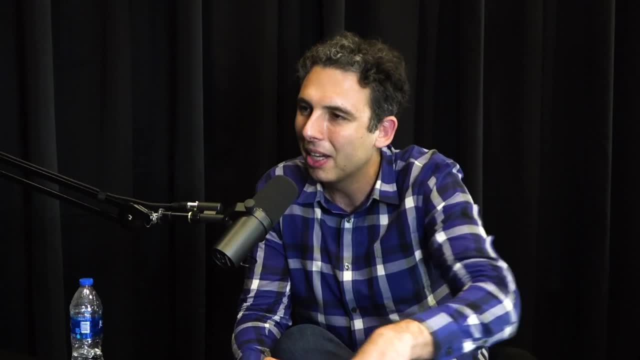 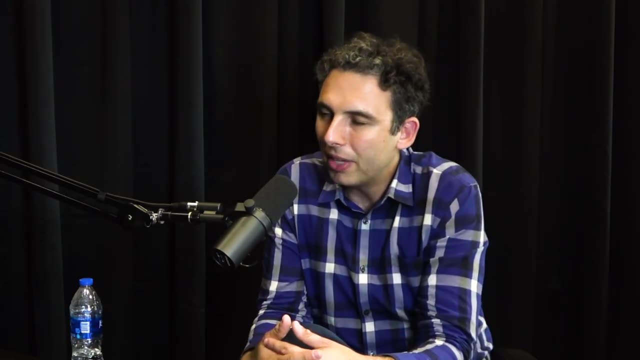 there's that, there's like caching and like, And there's like a really reasonably well established modularity and APIs and so forth, And so you can kind of like scale it in an efficient fashion. That doesn't exist anywhere near to that level of maturity in autonomous driving right now. 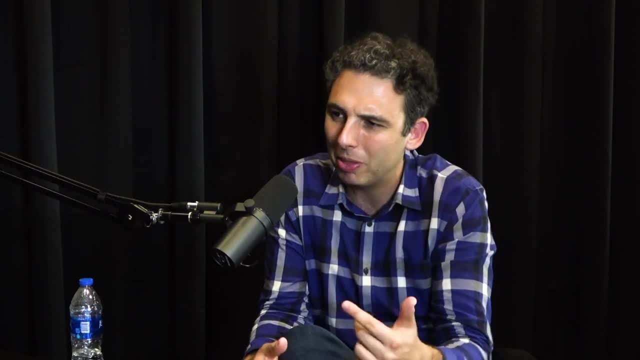 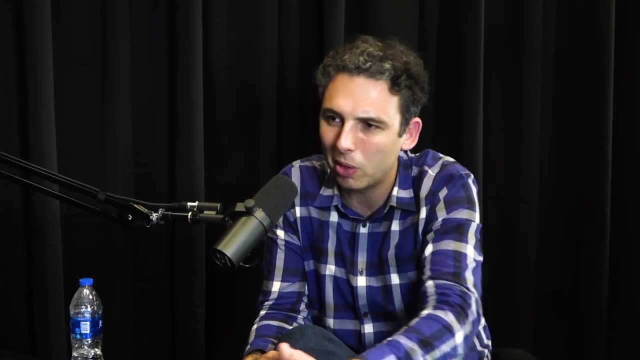 And tech stacks are being reinvented, Organizational structures are being reinvented. You have problems like pedestrians that are not isolated problems. They're part sensing, part behavior prediction, part planning, part evaluation And like, one of the biggest challenges is actually: how do you solve these problems? where?